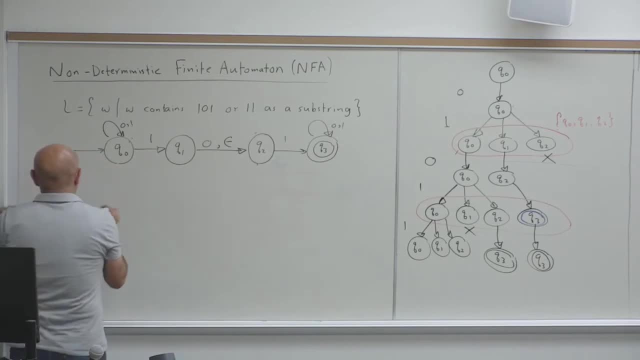 Okay, so the mathematical definition of a of an NFA non-deterministic finite automaton is a 5-tuple Q, sigma, delta, Q0 and F. In fact everything is the same except for delta, So Q is a finite automaton. 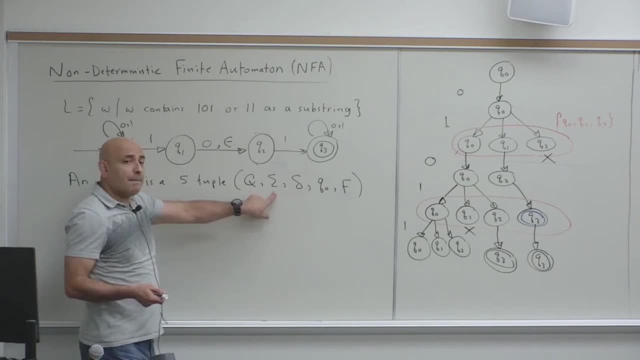 It has a set of states. Sigma is a finite set of symbols, Delta is what The transition function. Q0 is the start state, F is the final state And all definitions are the same except for the delta. Delta is the only difference between an NFA and a GFA. 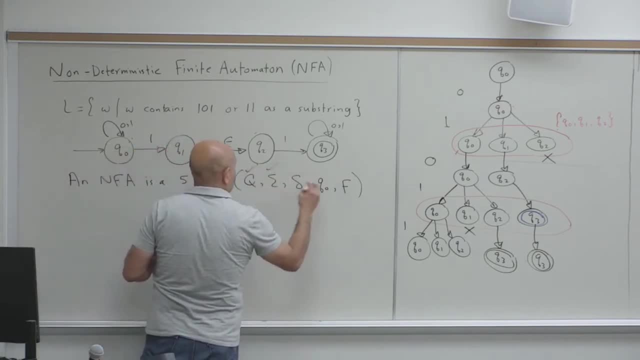 So for Q, Q0 and F is the same as the GFA, but for delta? Now let's try to think of delta. Now there is a domain and a range. What's the domain and what's the range for delta and an NFA? 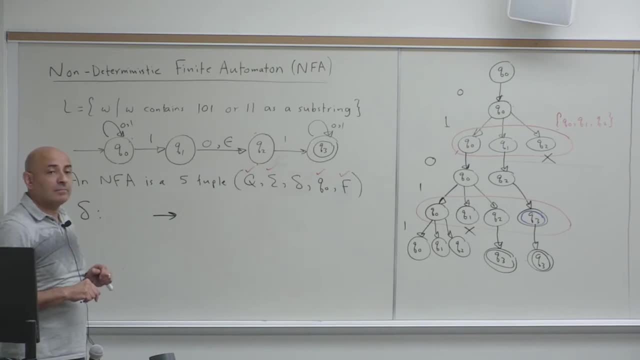 So what's the domain? So we have to add, yeah, we have to add the epsilon somehow. So in fact, you know, remember, for the DFA, the DFA was delta from Q cross sigma to Q. That's for the DFA. 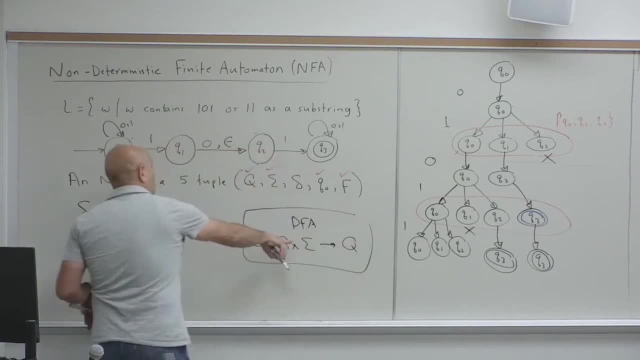 For a DFA we had from Q cross sigma to Q, But here it's not going to be sigma because we have epsilon transitions. So we will define that sigma sub epsilon As sigma union, the set that has epsilon in it. So we will add the epsilon symbol to the sigma. 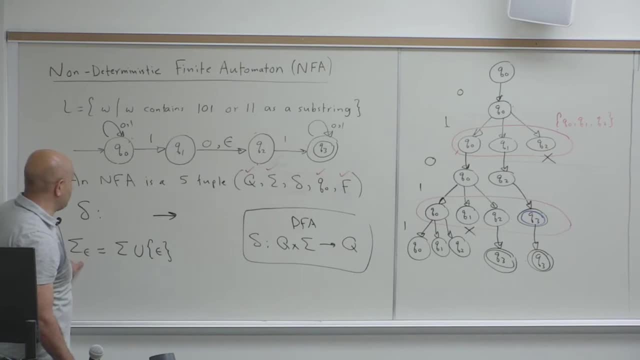 and we will define something called sigma sub epsilon. So that's going to be our domain for the NFA: Q cross by sigma sub epsilon And then what's going to be our range. So, before we think of it mathematically, think of it as a program. 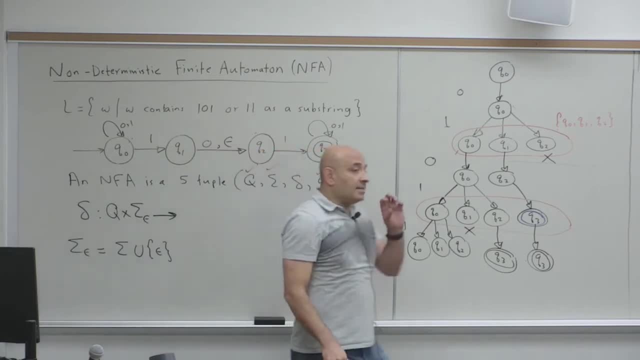 You have a program that implements a DFA. It takes a state and a symbol and it gives you what as output: State and symbol. Think of it as a function, not a program, Maybe a function. It takes a state and a symbol and it gives you a symbol. 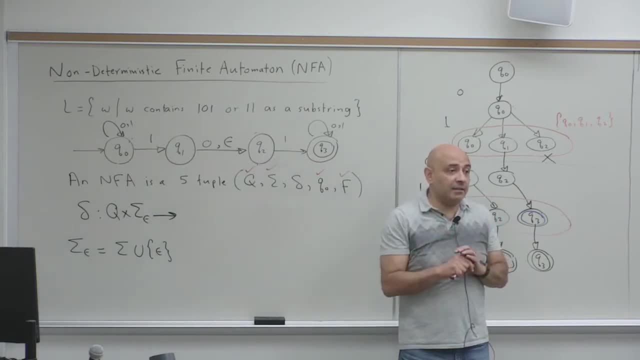 That's a transition. That's a transition function for a DFA. It takes a state and a symbol and it gives you a symbol. It gives you a state. Sorry, It gives you a state Now for the NFA. it takes a state and a symbol. 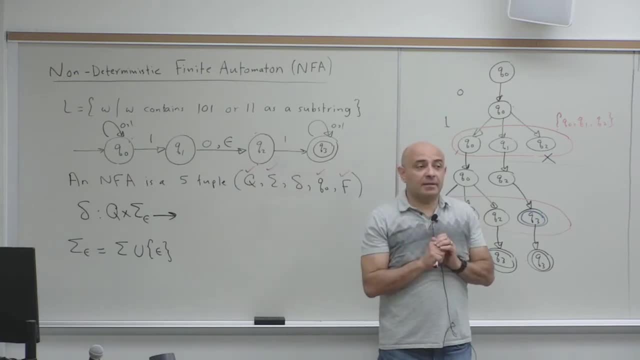 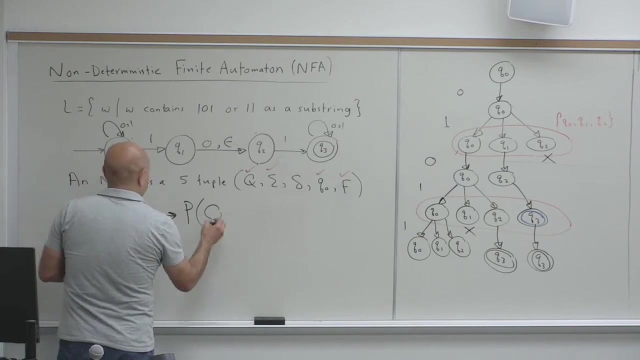 and the symbol can possibly be an epsilon. It gives you what Multiple states. Multiple states, Yeah exactly, It can give you multiple states. So it will give you a set of states, A set of states. So that's why the range for the NFA is the power set of Q. 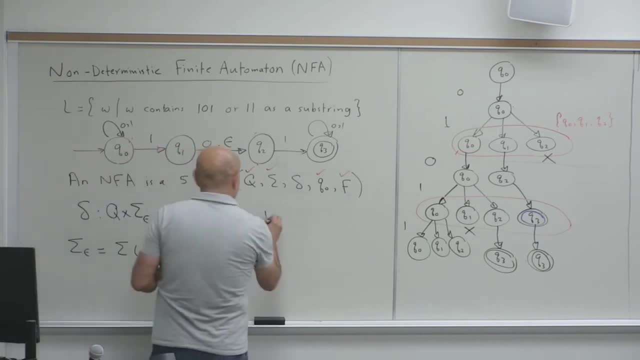 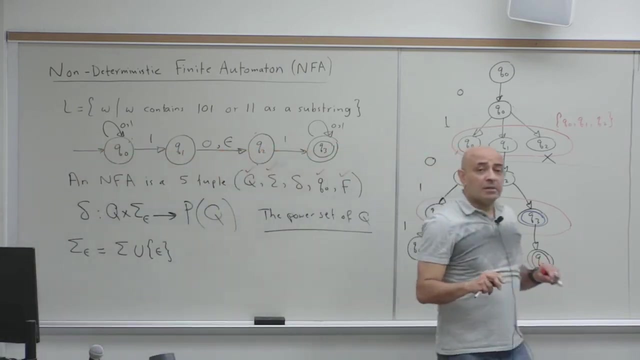 the set of states. So P of Q is the power set of Q. What's the power set? How would you define the power set of Q? What's the power set of Q? What's the power set of a set? It's a set of all sets. 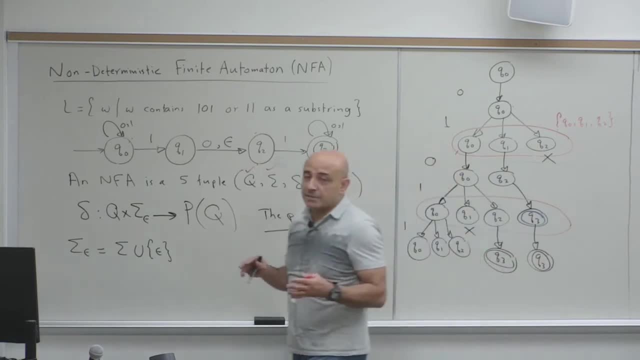 Yeah, exactly, It's the set of all subsets. That's what the power set is: The set of all subsets. Okay, So the transition function in NFA takes a state and a symbol that is possibly epsilon, and gives you a set of states. 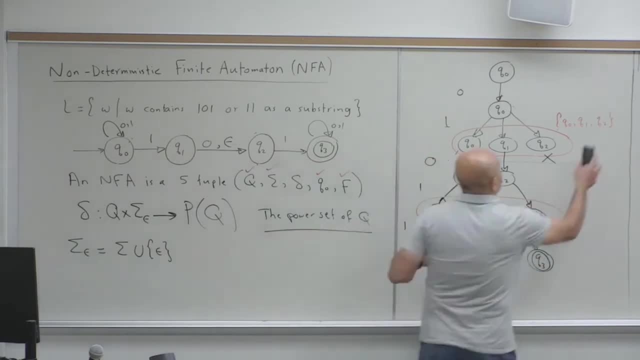 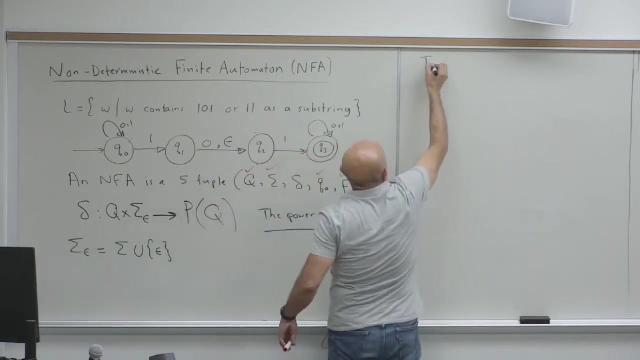 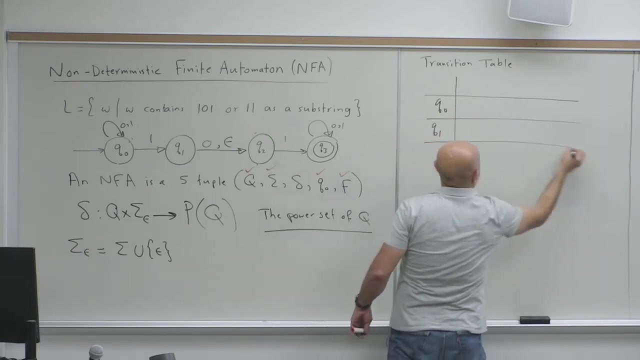 So let's apply it to this. So let's write the transition function of this energy In the form of a transition table. So let's write the transition table for this. So we will have a state Q0,, Q1,, Q2,, Q3.. 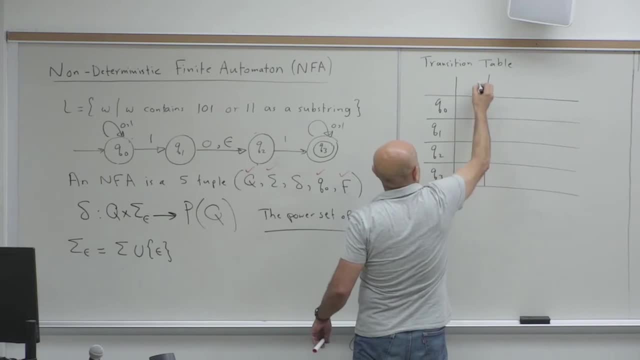 And we will have symbols 0,, 1,, epsilon. Okay, Now here, we don't trace You, just you, just you know, put the transitions that you have in the transition diagram, You put them in the table, That's all what you do. So, if you have a Q0,, Q1,, Q3,, Q4,, Q5,, Q6,, Q7,, Q8,, Q9,, Q10,, Q11,, Q12,, Q12,, Q13,, Q13,, Q14,, Q15,, Q15,, Q16,, Q17,, Q18,, Q19,, Q20,, Q21,, Q21,, Q21,, Q22,, Q21,, Q22,, Q23,, Q23,, Q23,, Q23,, Q24,, Q24,, Q24,, Q25,. Q26,, Q27,, Q29,, Q30,, Q31,, Q32,, Q36,, Q37,, Q40,, Q40,, Q41,, Q42,, Q46,, Q44,, Q45,, Q46,, K48,. 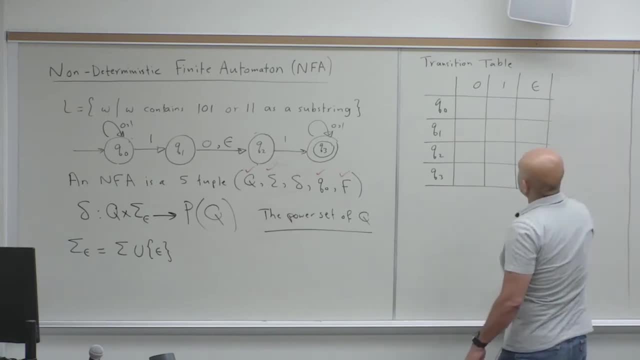 Q49,, Q50,, K51,, K52.. Now here we don't trace You, just you. just you know, put the transitions that you have in the transition diagram, You put them in the table, That's all what you do. 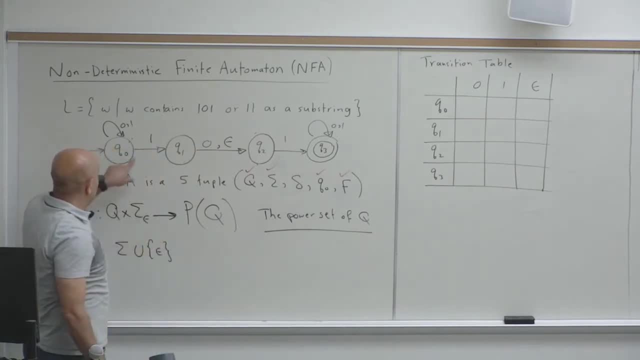 So if you have a Q0 and you get a 0. You stay Q0, but it's the set Q0.. So it's a set of states that happened to have only Q0 in it. If you have a Q0,, Q10,, Q11,, Q12,, Q14,, Q13,, Q14,, Q15,, Q16,, Q13,, Q14,, Q15,, Q14,, Q15,, Q14,, Q12,. 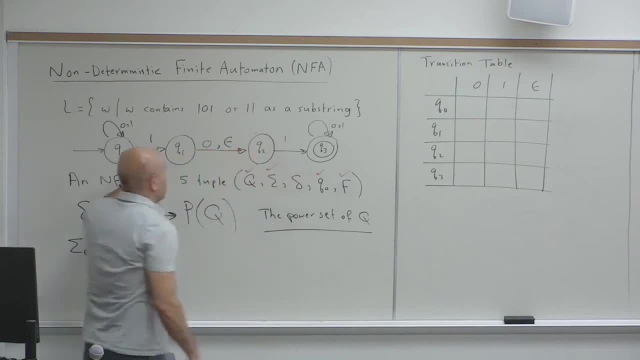 You just, you know- put the transitions that you have in the transition diagram, you put them in the table. That's all what you do. So if you have a Q0 and you get a 0, you stay in Q0,. 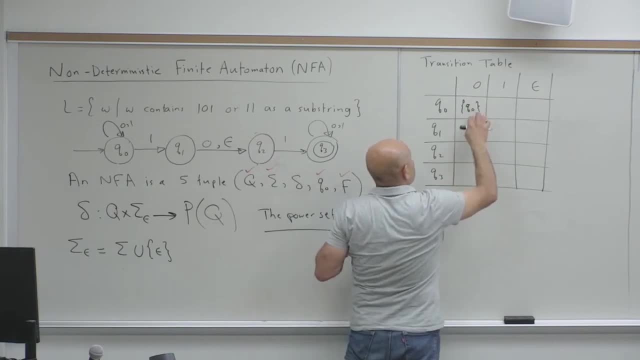 but it's the set Q0.. So it's the set of states that happen to have only Q0 in it. If you are in Q0 and you get a 1, where do you go? Yeah, Q0 or Q1.. 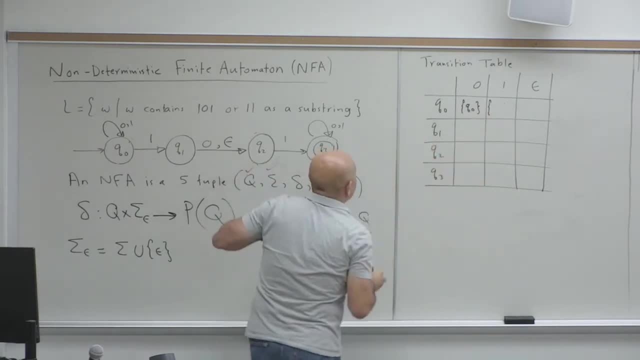 So now we're not tracing, So we're not going to say Q2 here because we're not tracing. now We did that when we traced. We're not doing actual tracing, We're just, you know, translating what's in the diagram. 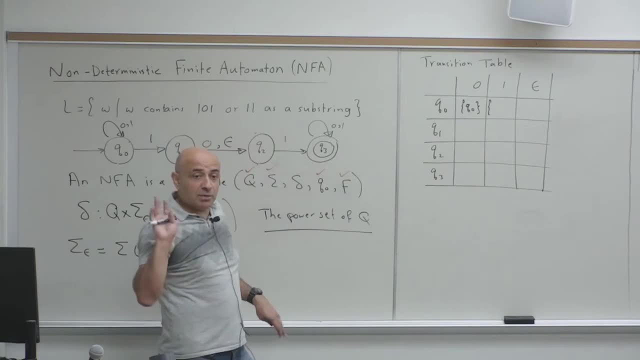 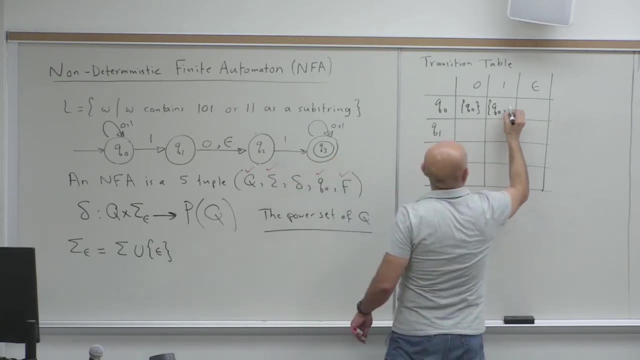 into a transition function in the form of a table. So we're just translating, We're not tracing Q0 or Q1.. Okay, If I'm in Q0 and I get an epsilon, where do I go? There is no epsilon transition out of Q0, so I go to low state. 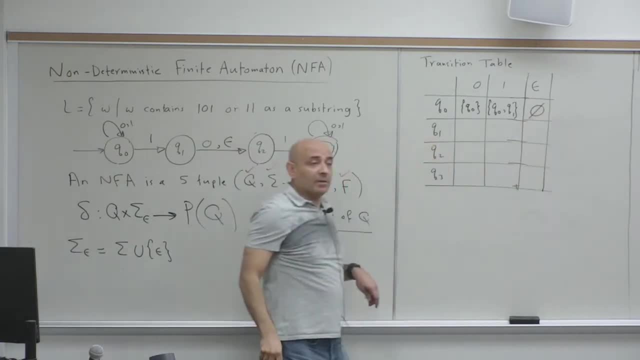 and that's the empty set of states. Okay, So this is, it goes to an empty set of states. Yeah, So it's not an implied epsilon transition to yourself And implied no, because on no input you could always stay in the same spot, right? 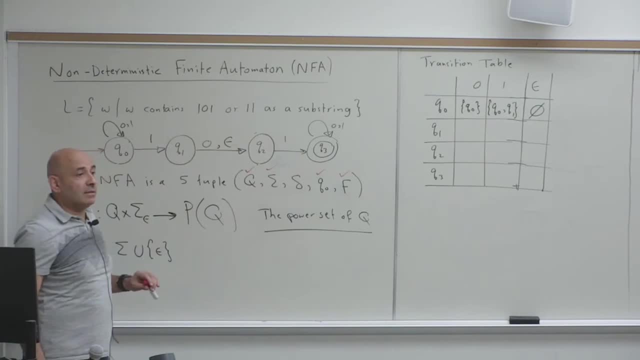 Okay. So again, this is: you are tracing, You are not translating. We're translating the transitions that are in the diagram. What we are doing now is a translation, not a trace. Okay, So yes, I mean, but what does it mean? 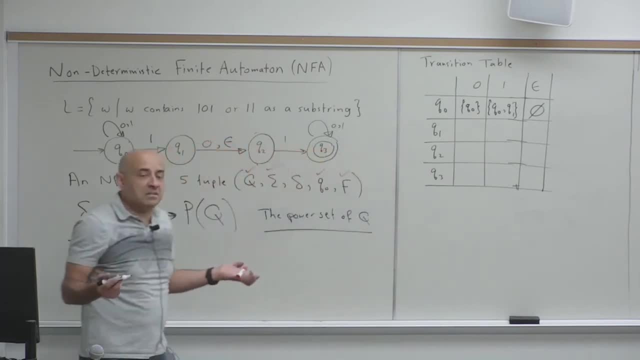 I mean, if epsilon transition to yourself, what does that mean? It means you just say, oh, I'm in Q0.. It means you just stay in the same state. But that's a tracing thing, not a translation. Now, Q1, if I get a zero, what happens? 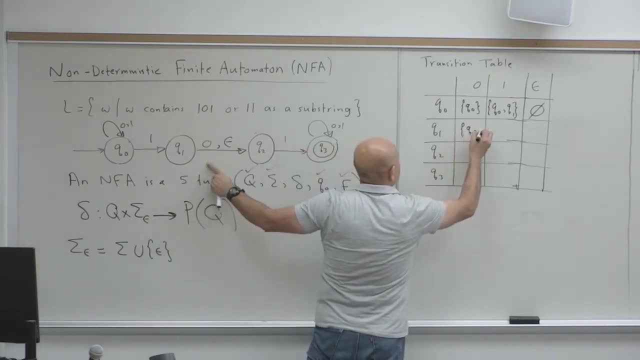 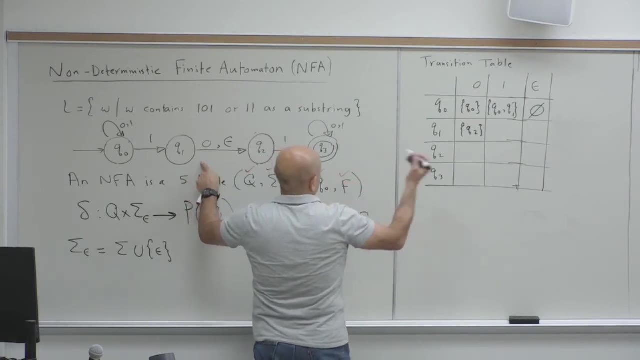 You go to Q2.. Q1 and you get a one: Okay, Nowhere. Yeah, Q1 and you get an epsilon. you go to Q2.. Q2 and you get a zero: nowhere. If you get a one, you go to. 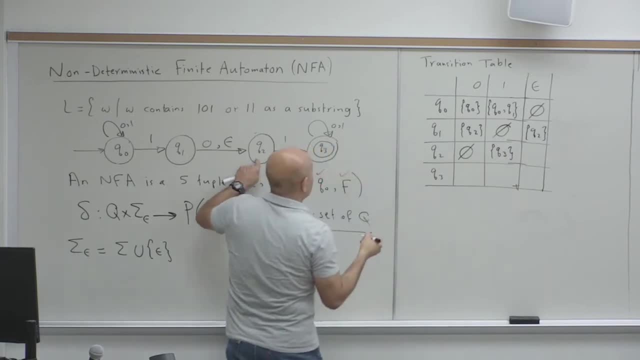 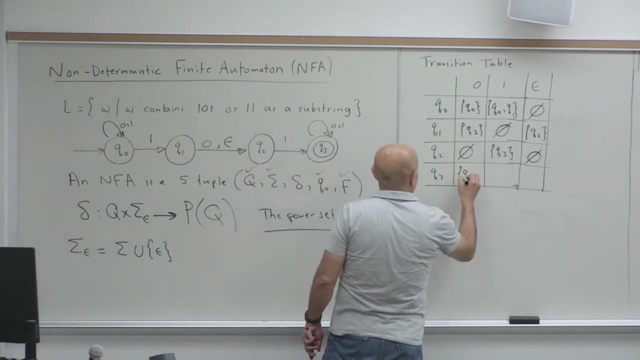 Q3., Q3.. If you get an epsilon, nowhere And Q3, you are in Q3.. If you get a zero, Q3.. Yeah, You go to Yeah, Q3. Q3. And if you get a one, you also go to Q3. 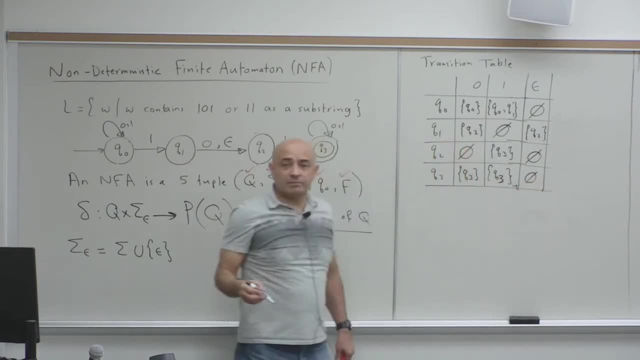 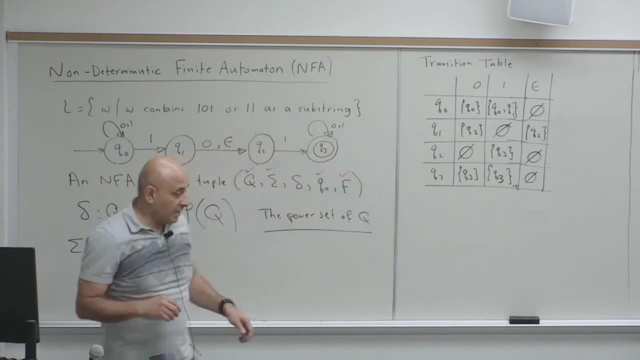 And there is no epsilon transition. Okay, Questions on this. Oh, so keep in mind that the idea is an NFA takes you from one state to a set of states, All possible states That you can go to And in general, you know, you can have multiple states. 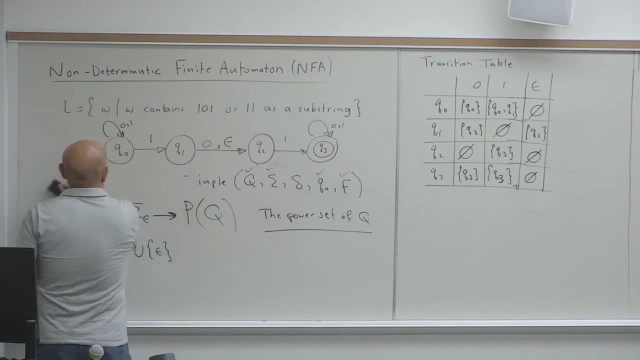 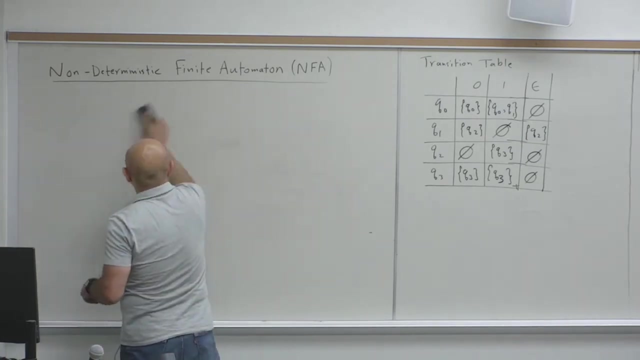 or you can have no states. So let's take another example. You see the power of. In fact. in fact, for the same language, there is always a standard way. I'm going to do it again. W is that W contains 101 or 11 as a substrate. 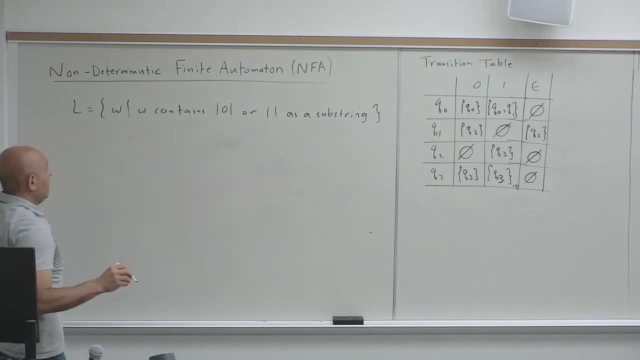 For this language. in fact, I could have drawn the DFA, the NFA. There's a standard way of constructing an NFA for a language that has an or in it. It's the or of DFA. We'll say more about this later. 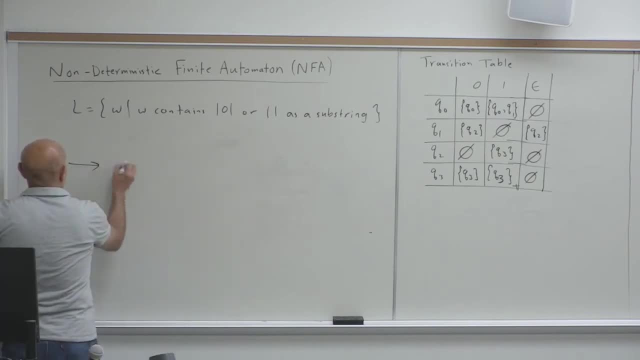 But we have an or. You can always say, okay, this is my start state, And then I have two possibilities Because of the or, So and I can do it. two possibilities with epsilon transitions. Then I can draw an NFA for the language that has this. 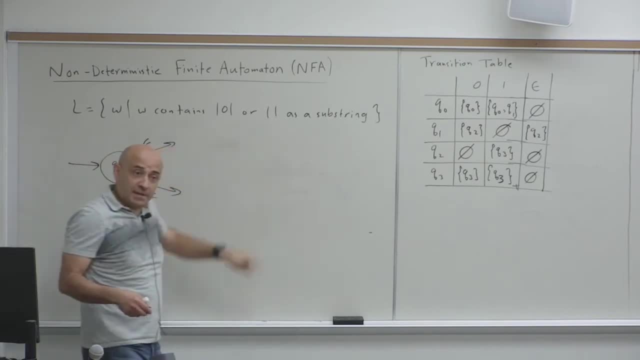 as a substrate and an NFA for the language that has this as a substrate, And that's all what I need. So I can say: for this as a substrate, this is a substrate, Then it's going to be this 101 and then this: 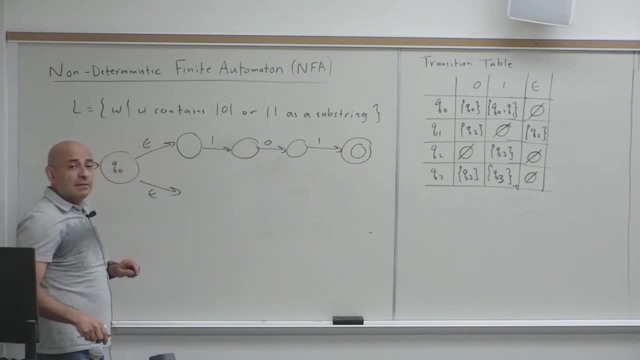 And before the 101, I can have anything. How do I express anything? No, How do I express anything here before the 101?? Yeah, looping on a zero or a one, So anything, it means anything before this string that I'm trying to match will keep you in this state. 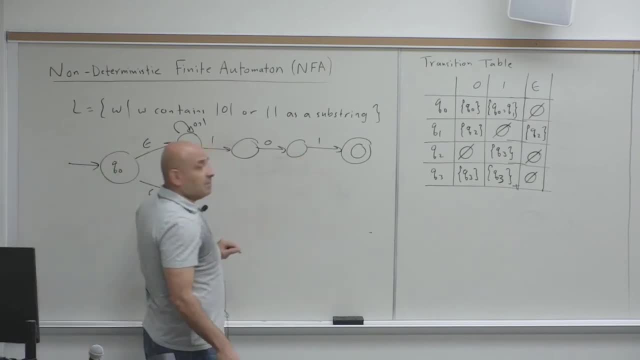 So if you get a thousand symbols before the symbol that you're trying, the string, the substrate that you're trying to match, you stay there, And after this you can have anything too. And same here: one, one, two, three, four, five, six, seven. 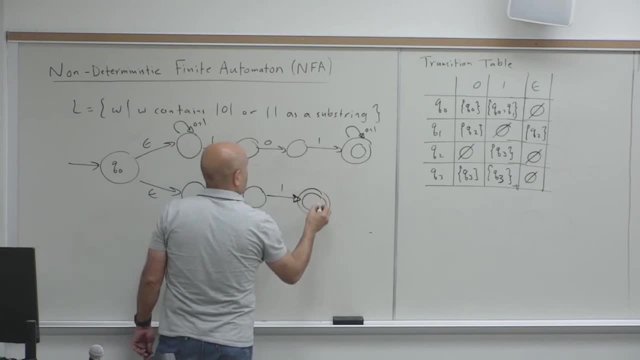 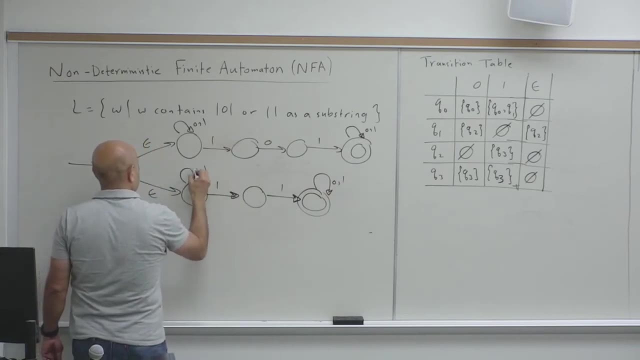 eight, nine, ten, eleven, twelve, thirteen, fourteen, fifteen, sixteen, twenty, twenty, Anything, Anything. So once you get used to the NFA it will be easy to use. So here I'm basically specifying in the NFA. 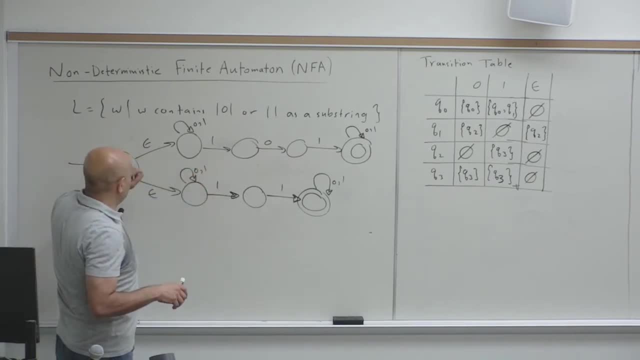 what I'm specifying is: you know what's a good path? Basically, I'm focusing on the good path And I'm implicitly rejecting. It's like I'm implicitly, without specifying anything. there is something that is not specified I'm rejecting. 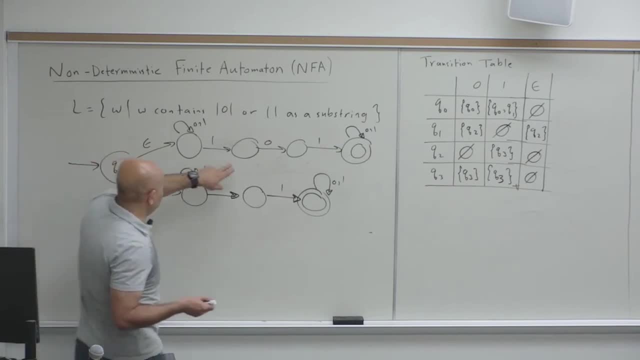 So you know, for example, if a string does not have 101, it's like the string you know 0, 010.. For the string 010, this will be rejected. How will it get rejected with this NFA? 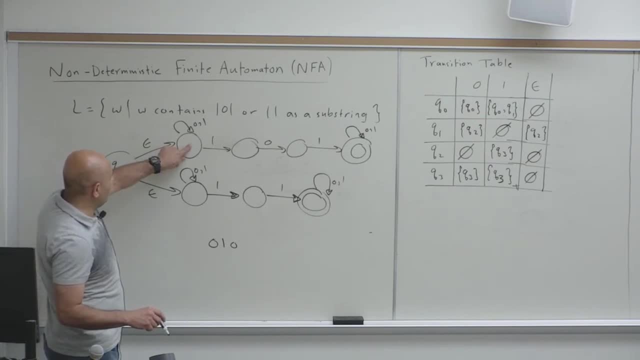 So: 0, you stay here. The 1, you have two possibilities: either stay or go to this, Whether you are here, or you are here when you get a 0, it will not take you to an accept state. 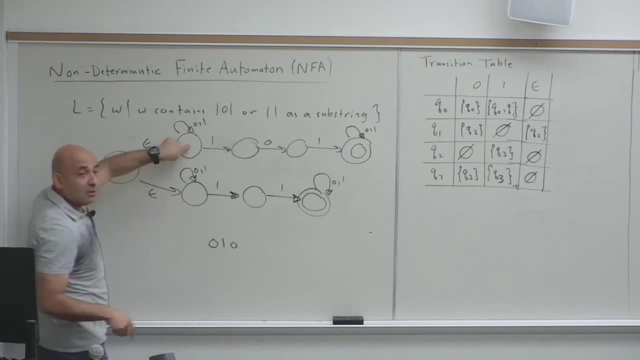 So for 010, the 0, you stay here. With the 1, you are either here or here. So you have two possibilities, But with either possibility the 0 will not take you to an accept state right. 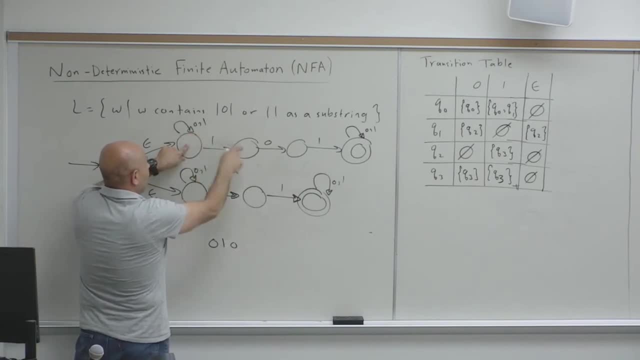 So this 0 takes you to keeps you in this state, and this 0 takes you to this, and neither one is an accept state. So when you construct an NFA- and you will get used to this- when you practice more basically you focus. 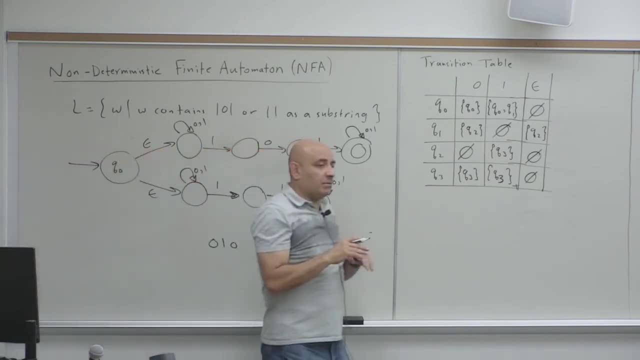 on what gets accepted and you don't have to think much about what gets rejected. It will automatically get rejected If you do it right, but you will get used to it And you will not have to do all the tracing that we did here. 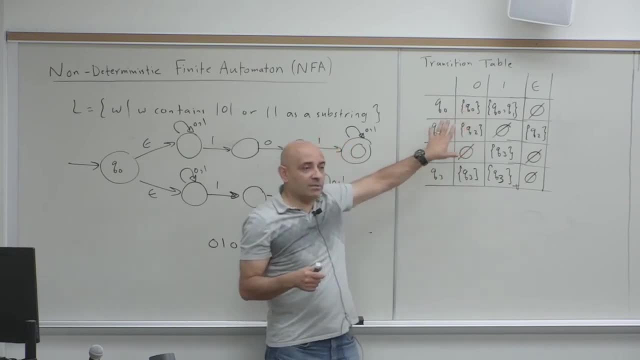 So you'll be doing it in your head. So this was done only once. We did it only once so that you understand how the NFA works, But from now on you will do that tracing in your head, Okay, Does anyone have questions? 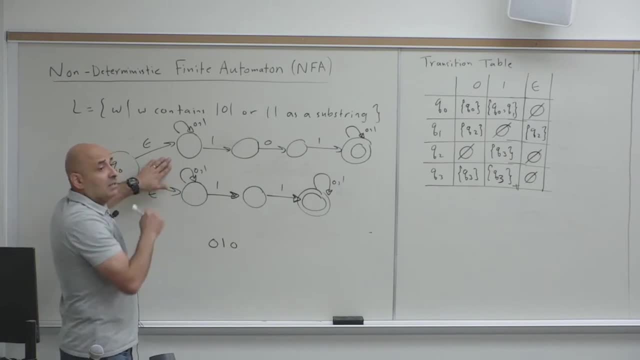 So this NFA is equivalent to the NFA that we traced. It has more states in it. That's the disadvantage, But what's the advantage? Yes, You tracked all the possible paths with the epsilon. No, they're equivalent. 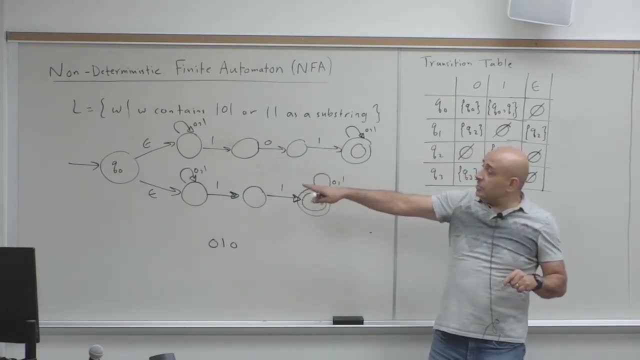 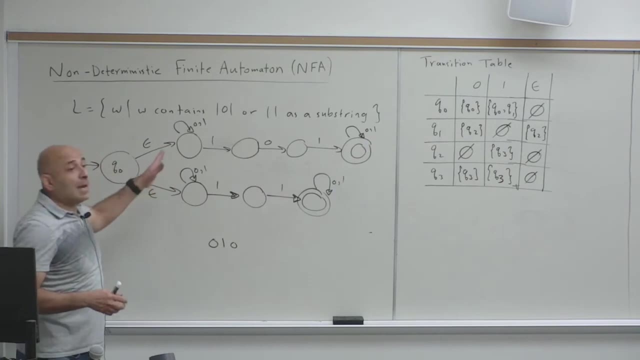 You know both NFAs are equivalent. The advantage in drawing the NFA like this is that this is more systematic, So you can do this. you can use this approach to construct an NFA for any tool that you want. Okay. 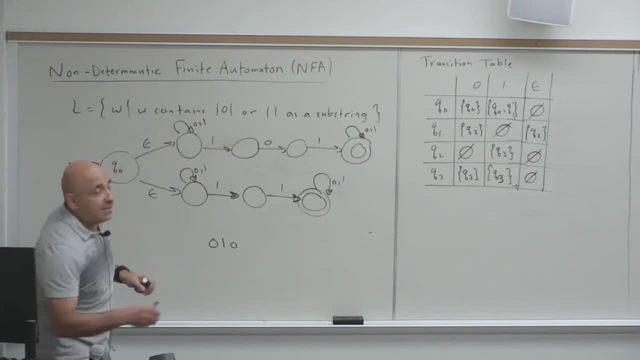 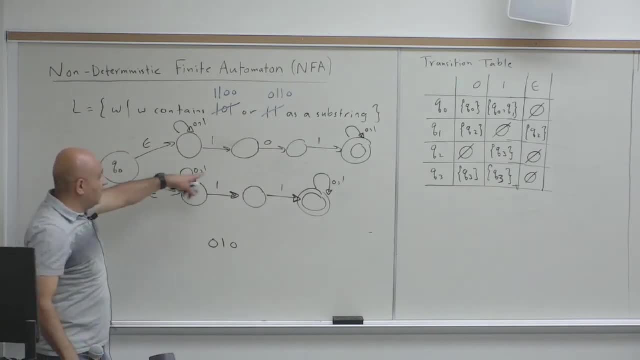 one one zero, zero and zero one one zero. you'll still be able to write an NFA this way, So you branch on epsilon and then you'll do an NFA for this and an NFA for this. 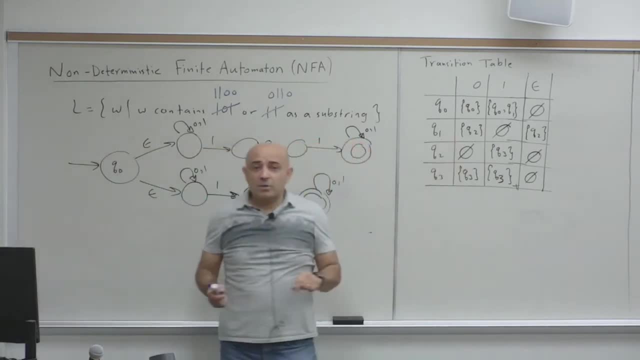 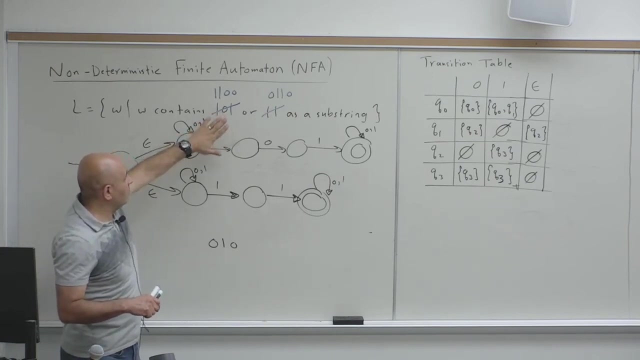 And that's all what you need to do. But the way we did it before, the one that we traced, was not general. it approach of strings. This is general to handle the approach I'm talking about, the approach. This approach is general enough to allow you to draw DFA. 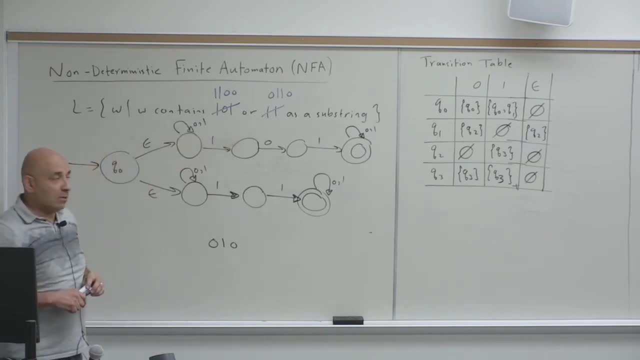 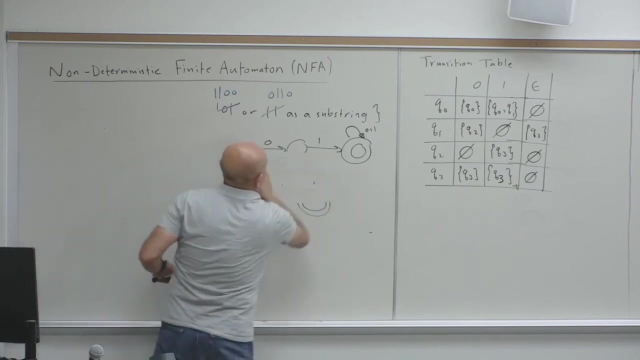 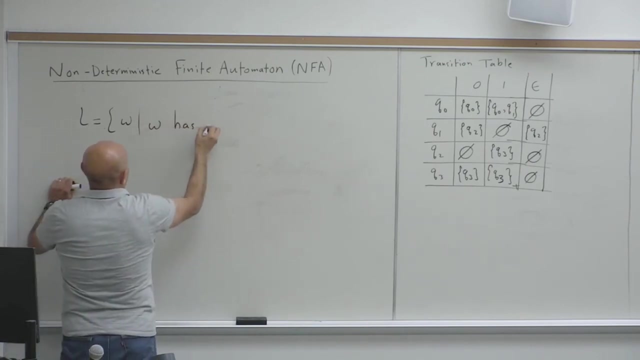 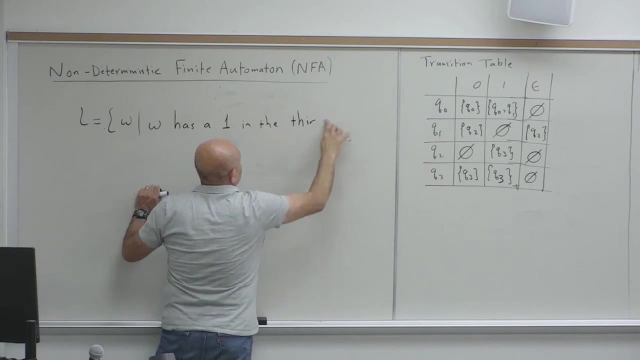 for any pair of strings or substrings. Okay, questions. Okay, let's do a quick one now. L is the language of strings W, such that W has a 1 in the third position. Has a 1 in the third position. 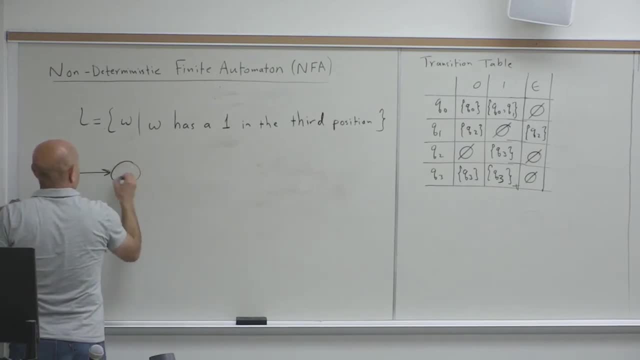 So that's easy. So what you do with an NFA? okay, so I have a 1 in a third position. So this is my third position, I have a 1.. So what should I have in first and second positions? 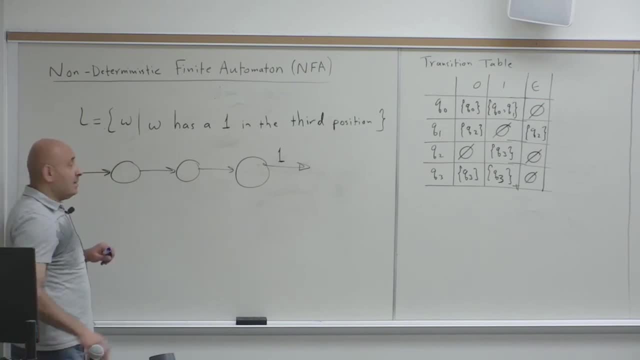 Absolute, Absolute, Zero. Anything, Anything is 0 or 1.. So I have, in the first position, I have a 0 or a 1. And in the second, I have a 0 and a 1, or a 1.. 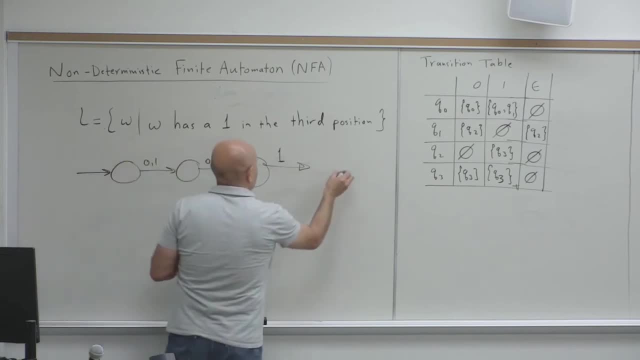 And then in the third position I specifically have a 1.. Then I have what I'll look for all of them. Yeah, for anything. So this is: W has a 1 in the third position. So I specified the third position. 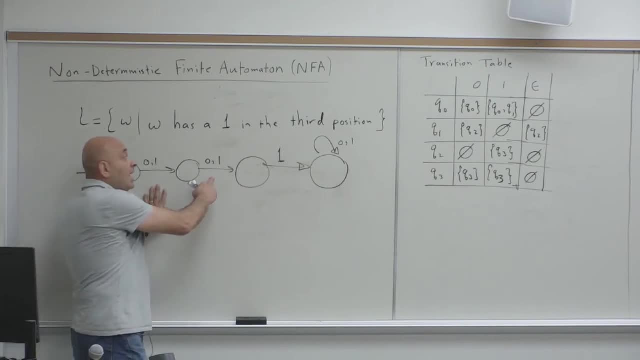 And before it I can have anything, After it I can have anything, And you know I didn't have to worry about you know here, for example, what happens if I get a 0. I didn't have to worry about this. 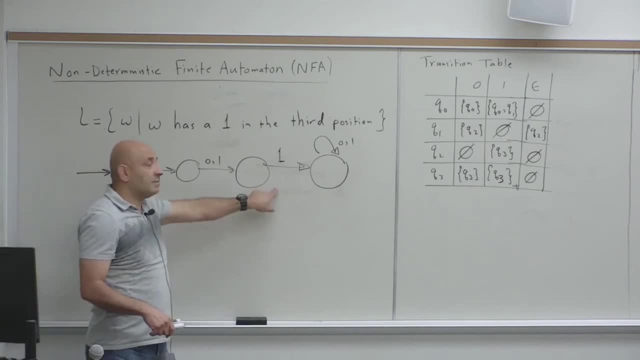 It's an implicit reject. If the third position is a 0,, this will be an implicit reject because it's going to lead you to a dead end. If your third symbol is a 0, you'll necessarily go to this. Then you'll go to this. 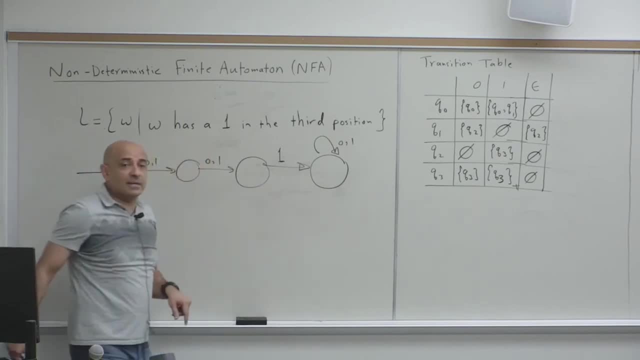 And if your third symbol is a 0, you'll nest There's an implicit reject, So the NFA basically implicitly rejects. Rejection is like implicit: You're not explicitly specifying it And that's why it's easier to construct. 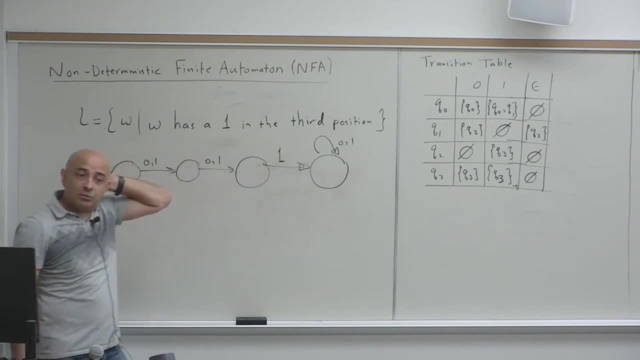 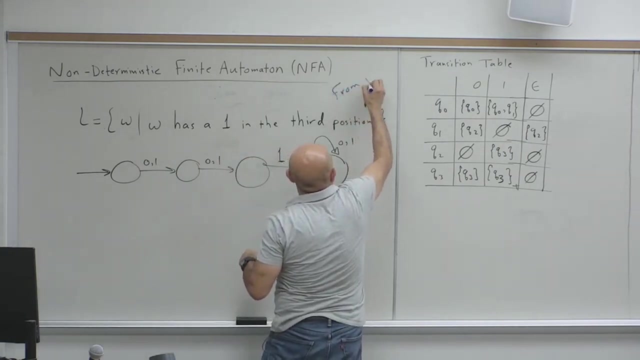 Once you get used to it, it's easier to construct than a DFA. You don't have to worry about everything. Okay, Now what if I change it? W has a 1 in the third position from the third position. So the third position from the N, Third position from the N. 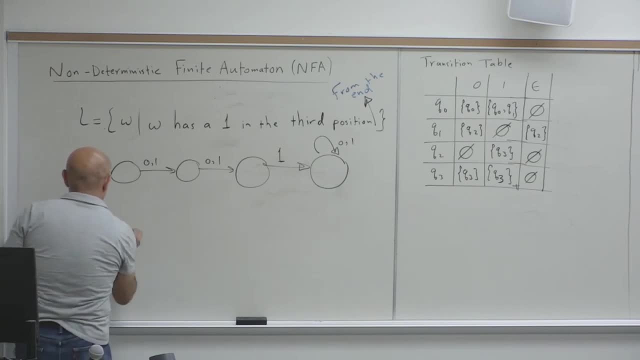 So the third position from the N. So I just did the one here, So let me do it in blue, because I did this in blue. So all that you do is Now I want the third position from the N to be a 1.. 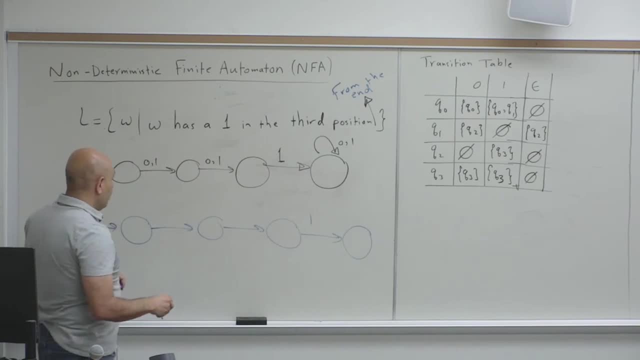 And then, before that I can have anything, Is this complete? Sorry, this is. Oh, this is an accept, But I forgot to put the accept state here. So this is the accept state. So what's missing? 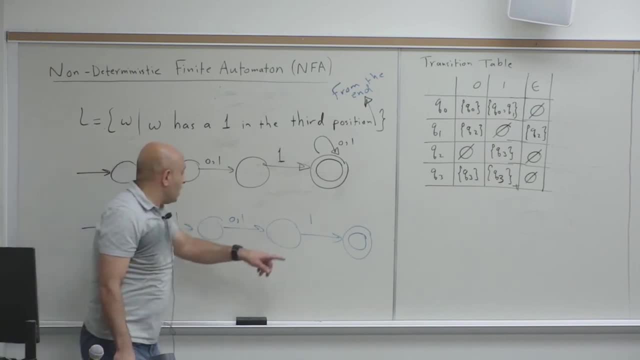 Who can make this correct? The third position from: Oh, so this is not the third position, Sorry, No, it's not. This is the last, So it's the other way around. So this is the third from the N, Then 0 or 1.. 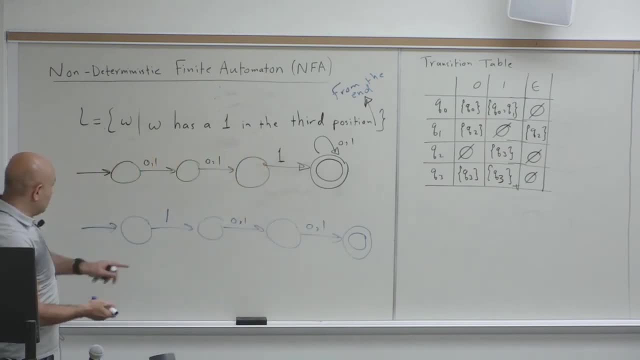 Then 0 or 1.. Sorry, So this is the third position from the N, Followed by anything, anything. Now what's missing? It needs to loop on itself at the state right before the 1.. Yeah, exactly. 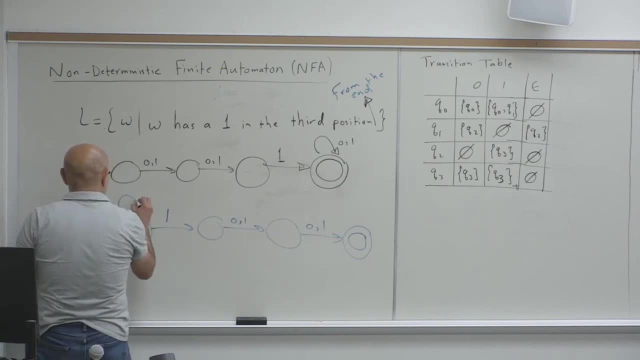 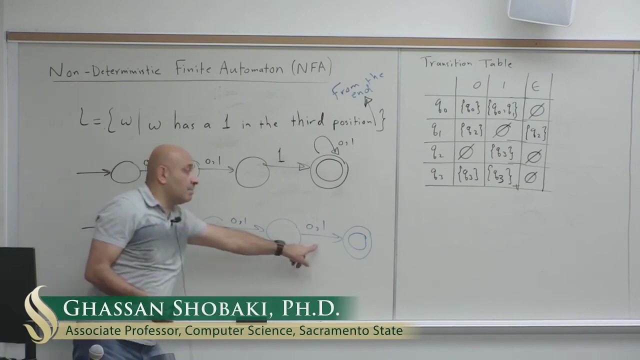 So in the beginning I can have anything. So in the beginning I can have anything. Then the third from the N is a 1. Followed by anything, anything. So I'm not specifying. you know what the third symbol is.